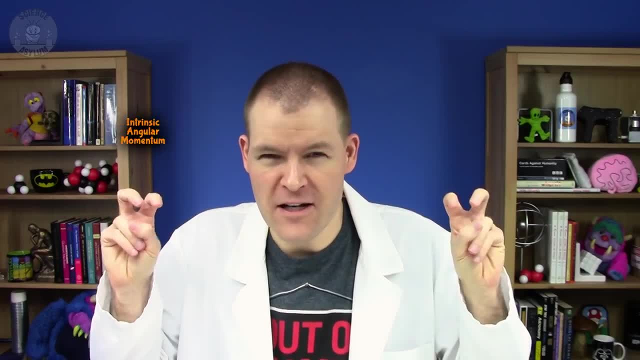 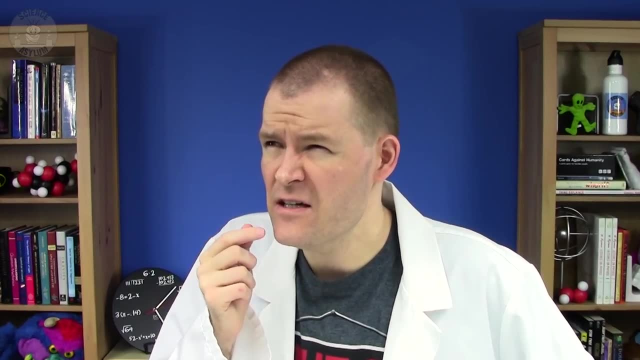 for no other reason It shouldn't even be called spin. Intrinsic angular momentum would be more accurate, but it's not nearly as catchy. Intrintum Intum Angtrinsic Tang Ugh. The reality is just so unfamiliar, there isn't a better word for it. 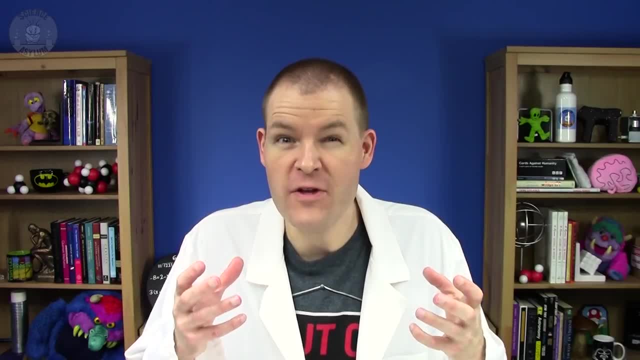 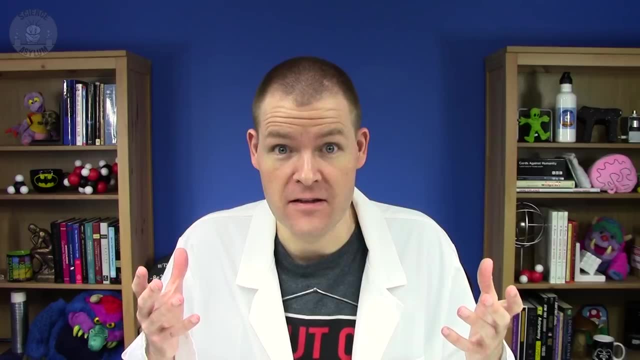 But how do we know it's there? Magnets: Any charge with any kind of momentum is going to have a magnetic field, which means it's going to be affected by a non-magnetic field- Magnets. We'll stick with electrons for now, because well, they're easy. 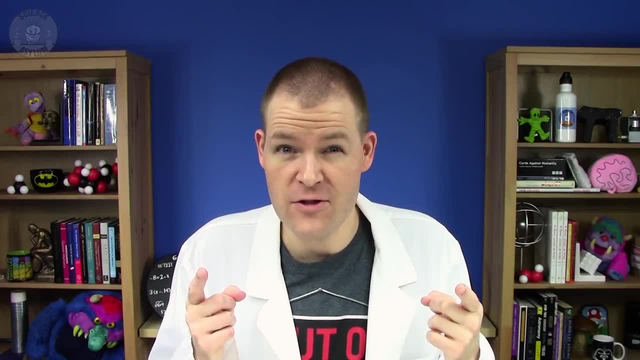 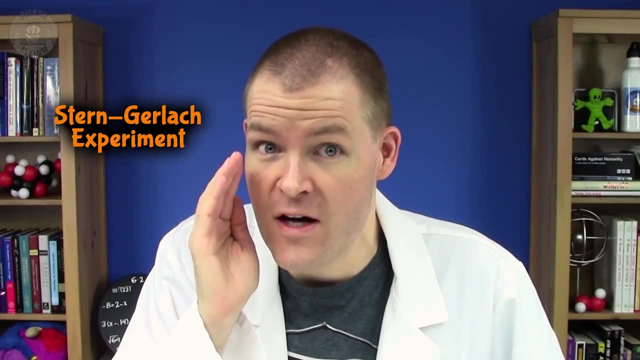 Experiment time. There was this experiment done in 1922, called the Stern-Gerlach experiment. Full disclosure. Otto Stern and Walter Gerlach did not use a beam of free electrons because that ain't going to work. Charge is a bigger influencer than spin, so they'll all veer off in the same direction. 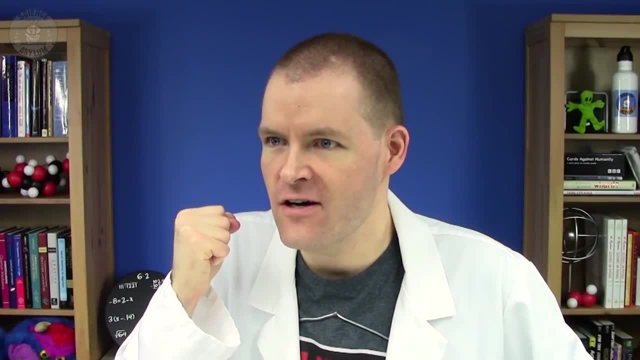 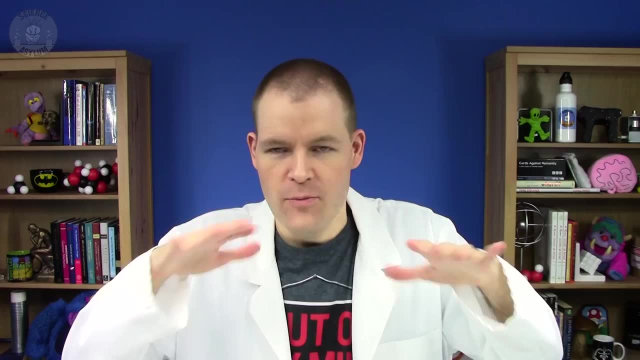 if they get too close to a magnet Charge. Such an attention hog. Anyway, you need to make it neutral like a whole atom. Stern and Gerlach used silver, cause reasons, But I don't want to get caught up in the details of the experiment. 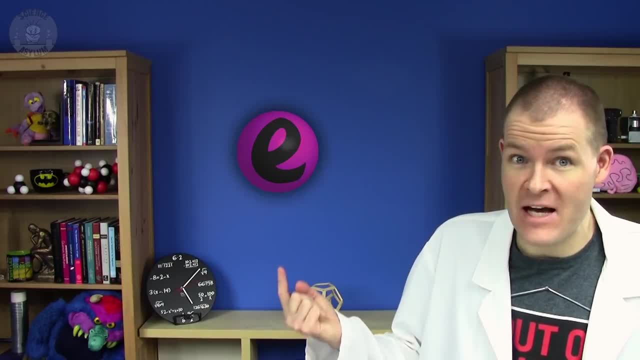 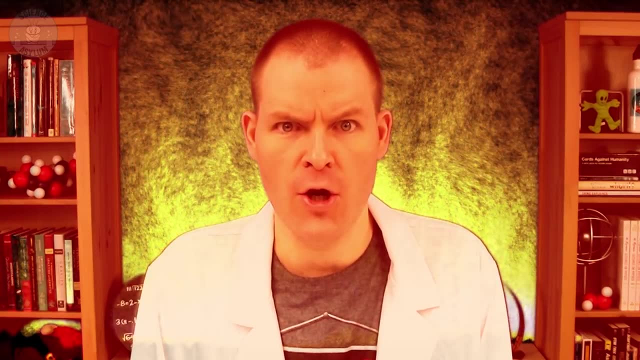 All that matters is we now have an atom that we're going to pretend is a massive neutral electron. I know it sounds silly, but that's how I feel about all experiments. Theoretical physics is superior. Next, we need something to control that electron. 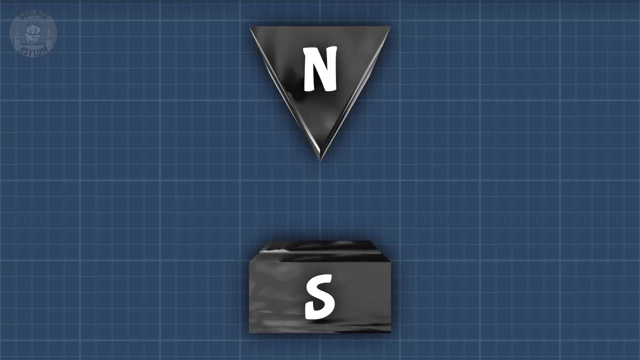 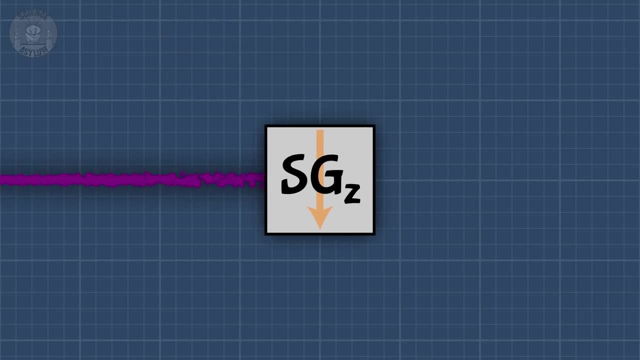 Say I don't know, two strong magnetic poles shaped like this. Again, don't get caught up in the details. Think of it as just a spin separator. If we send a bunch of these electrons through, we get two distinct groups, which we call. 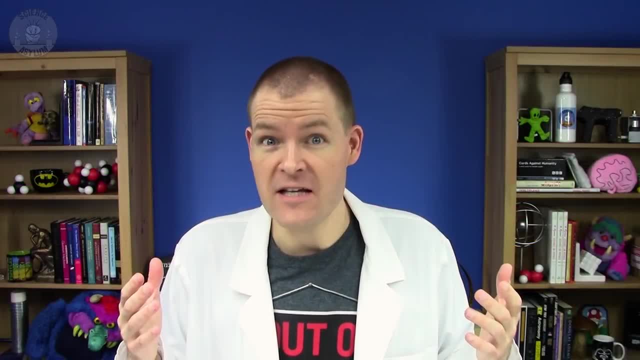 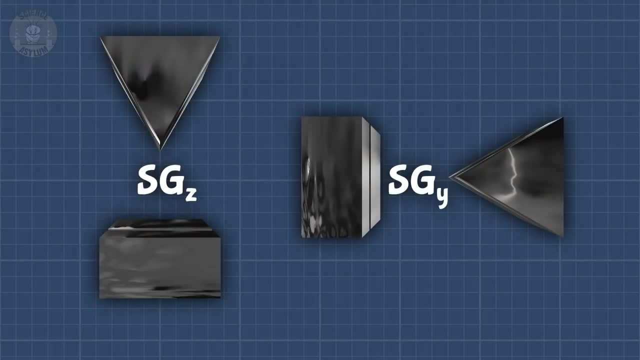 spin up and spin down. Since the biggest possibility is plus one half, we call these spin one half particles, But there's nothing special about up and down. We get two groups. no matter how we orient this thing, Each of the two major directions can only have two possible values: plus one half, and 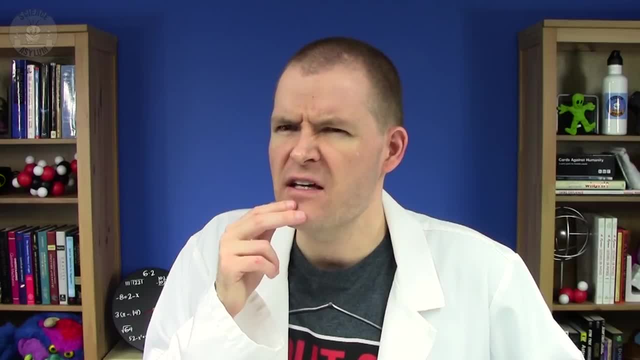 minus one half, Never zero. I wonder what that looks like If all the directions are plus one half. the spin arrow looks like this: I wonder what that looks like If all the directions are plus one half. the spin arrow looks like this: 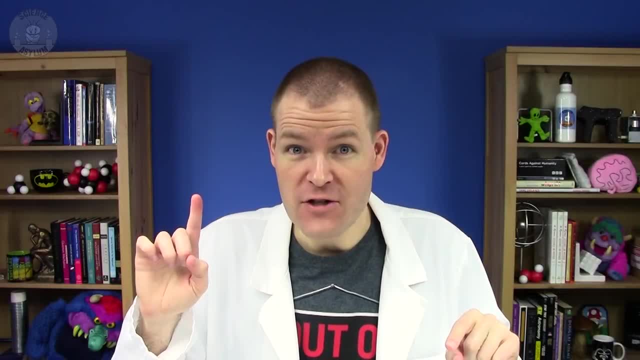 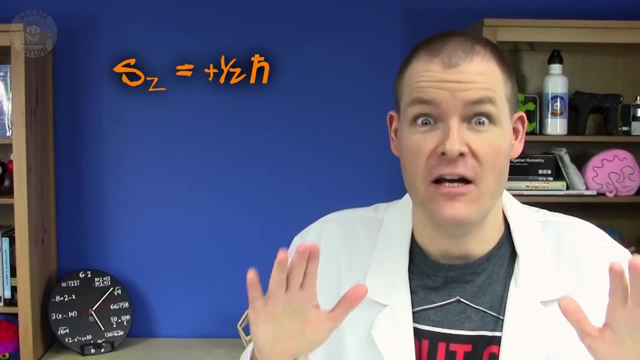 But this is quantum mechanics. Only one of those directions can be definite at any one time. What I mean is, if one of the directions is, say, definitely one half, like for sure, then the other two directions are in some weird combination of both plus one half and minus. 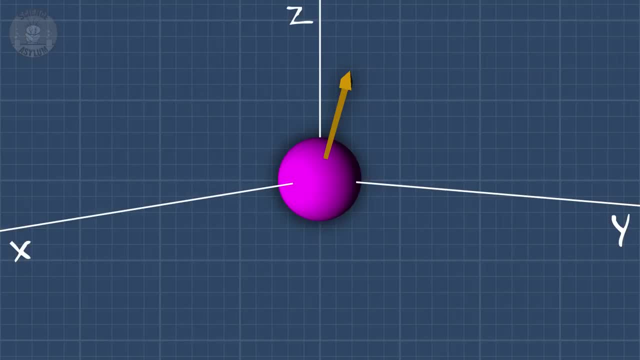 one half. It's called a quantum superposition, So spin up actually looks more like this: There are only four possible directions for that arrow, all pointed up. If we then try to measure left and right, We might find that it's pointed right, except now it's in this state. 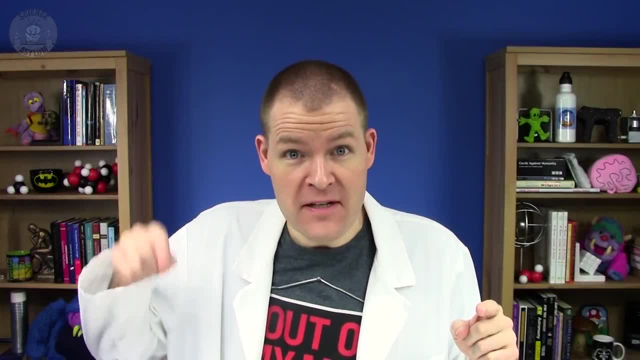 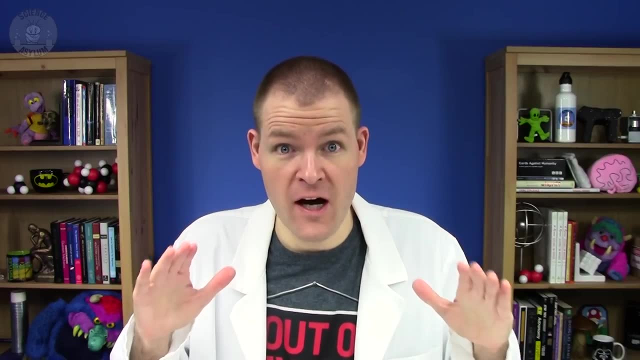 We don't know if it's up or down anymore. If you go back and measure up and down, you only have a 50% chance of getting up. I shouldn't have said that You only have a 50% chance of measuring up. 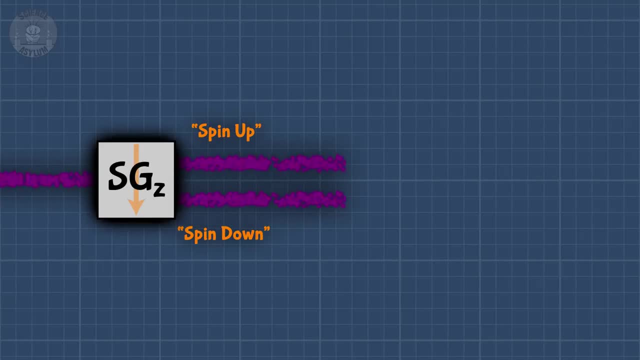 Ugh, now it's just depressing. I just mean that if you separate two groups in one direction, block one of those groups, then separate into two groups again in a different direction, block one of those groups and then remeasure in the original direction, you get two groups. Okay, Two groups, not one. It forgot the original measurement. There are always four possible directions to the spin arrow, so there is always quantum weirdness, Which is true of any spin one half particle, including protons and neutrons. Yes, neutrons. They might be neutral, but they're made of smaller particles that aren't neutral, so they're still tiny magnets. It gets even weirder with bigger spins. Spin one particles are separated into three groups, so their spin arrows would look like this: 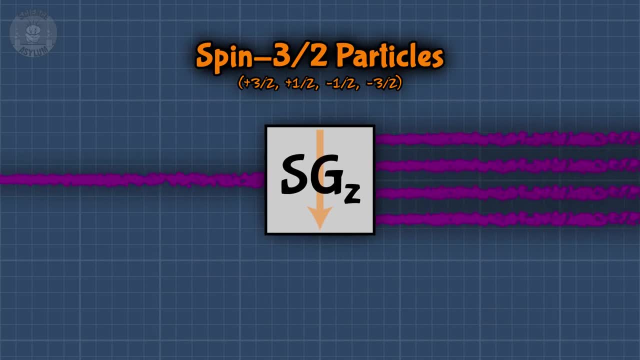 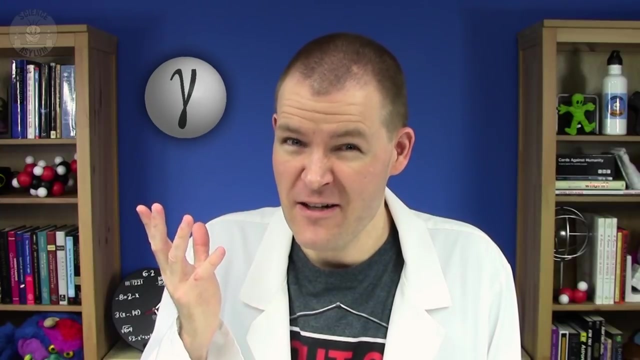 Spin three half particles are separated into four groups, so their spin arrows would look like this: Spin two particles are separated into five groups, and so on. Of course, this only works if the particle has charge on a fundamental level. If it doesn't like the photon, we have to be a little more creative. 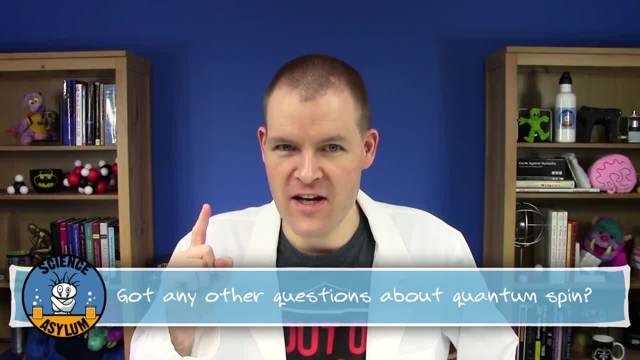 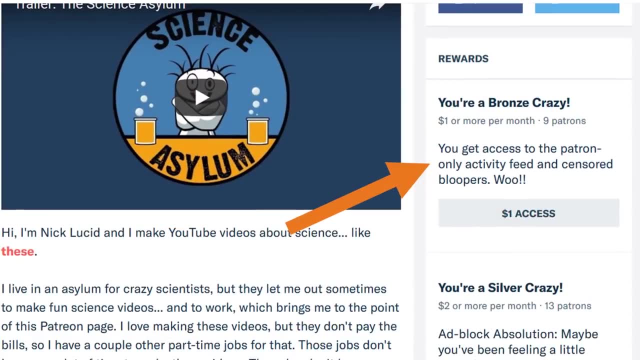 If you have any questions, please ask in the comments. Thanks for liking and sharing this video. Don't forget to subscribe if you'd like to keep up with us. Also consider supporting us on Patreon if you think we deserve it. Even one dollar a month can add up fast with enough people. 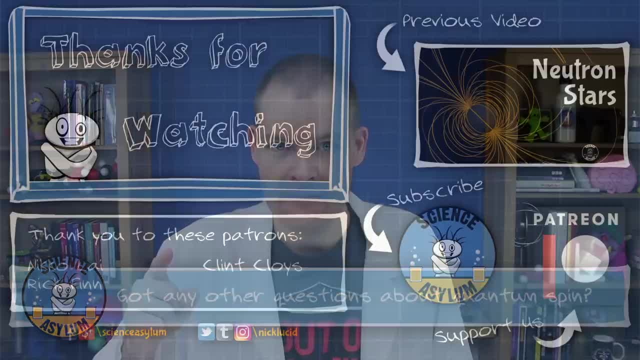 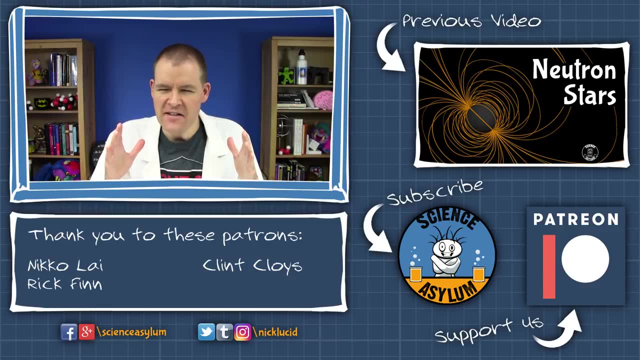 And until next time, remember it's OK to be a little crazy. The featured comment comes from SteveMonkey6666, who asked: Do neutron stars shine? Technically, yes, They are hot, so they are emitting light from their surface. 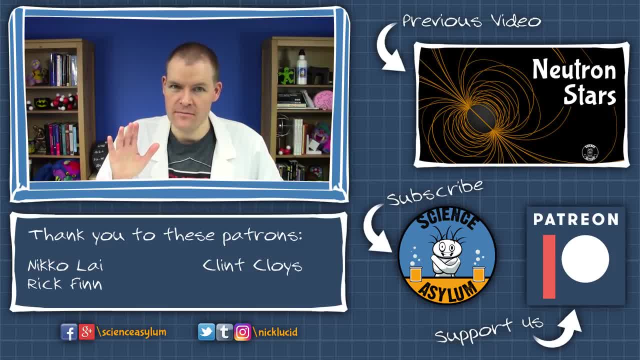 But they're not very bright. There's just not enough surface area. Thanks for watching. 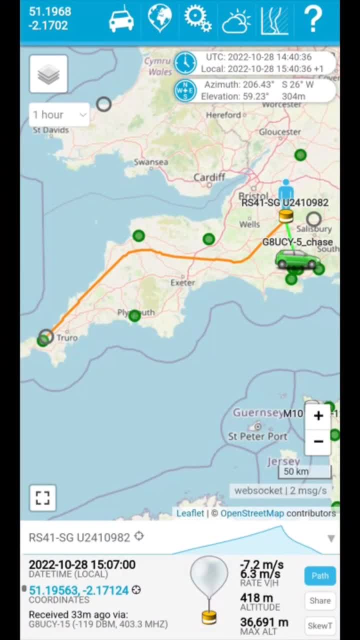 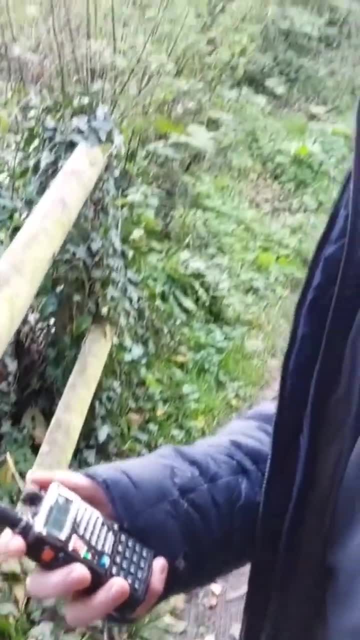 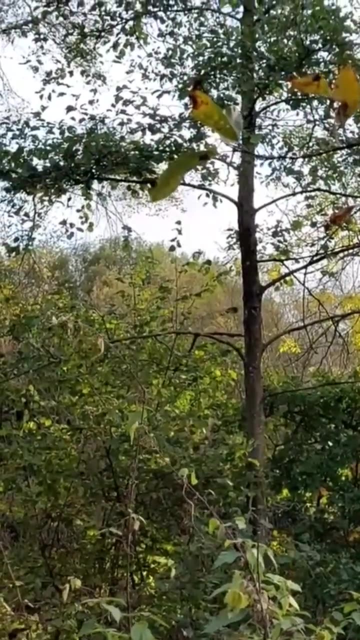 My aim for next year was to find and track one of these weather balloons but, as luck would have it, one was launched from Cornwall and blew this well. So we tracked it and it landed really close to where we were. so we jumped in the car and it landed in some private land on the edge of a. 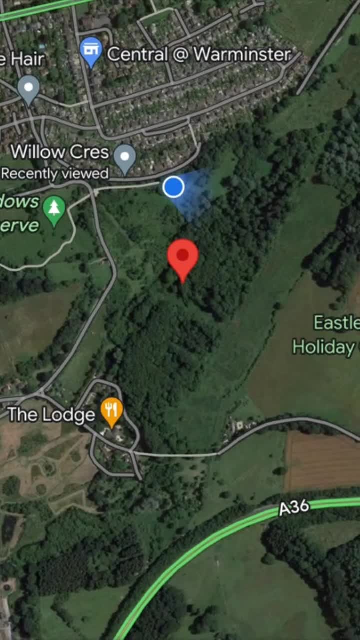 nature reserve, but we were so close this time and we could almost smell it.